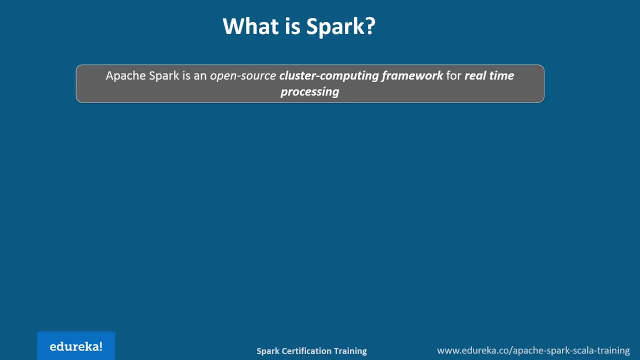 for real-time data processing. It is also designed for fast computation- The main feature of spark as its in-memory cluster computing that increases the processing speed of an application. Not only that, spark also provides an interface for programming entire clusters with implicit data parallelism. 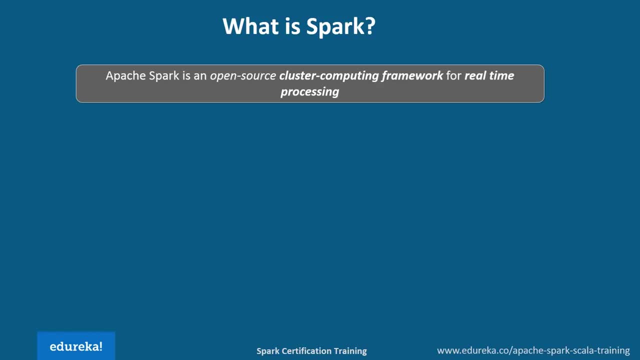 and fault tolerance. in this case, You do not need any special directives, operators of functions, to enable parallel execution. spark by default provides you data parallelism. Now let's see The various features of spark coming to speed. as you all know that it supports in-memory cluster computing. 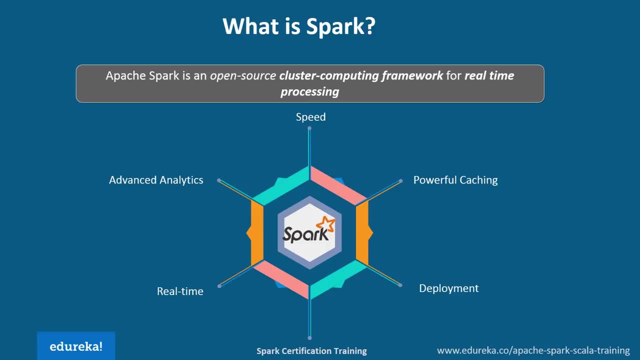 the processing speed of spark is 100 times faster in memory and 10 times faster in disk. next, powerful caching. spark is written in simple programming language and provides powerful caching and disk persistence capabilities. coming to deployment, spark supports well-defined user APIs that are written in Java Scala. 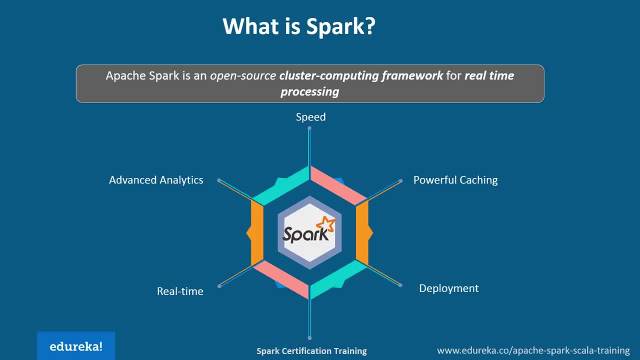 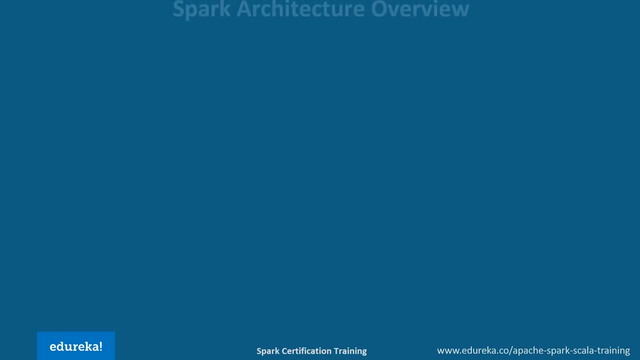 Python and it can be easily deployed in various platforms. As you all know, that spark itself was designed for real-time data processing, and it also supports advanced big data analytics like machine learning library, spark, SQL graphics and many more. Now let me just give you an overview. 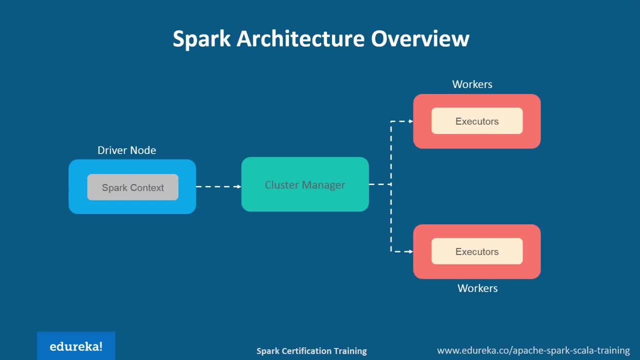 of the spark architecture. Apache spark has well-defined layered architecture where all the components and layers are loosely coupled and integrated with various extensions and libraries. This architecture is based on two main abstractions. first one, resilient distributed data sets, that is, RDD, and the next one directed a cyclic graph called DAG or DHE. 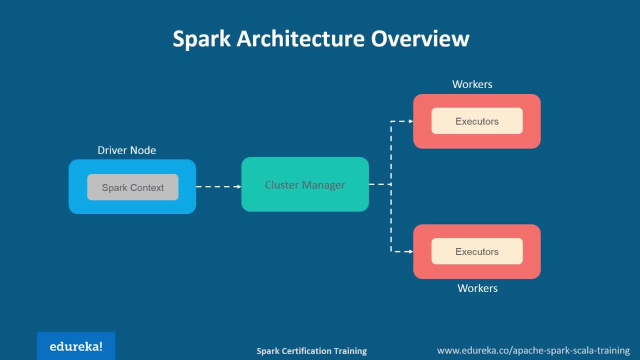 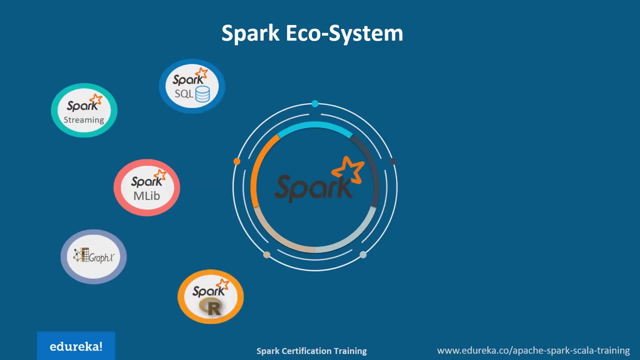 in order to understand this park architecture, You need to first know the components of the spark, that the spark ecosystem and its fundamental data structure, RDD. So let's start by understanding the spark ecosystem. as you can see from the diagram, The spark ecosystem is composed of various components. 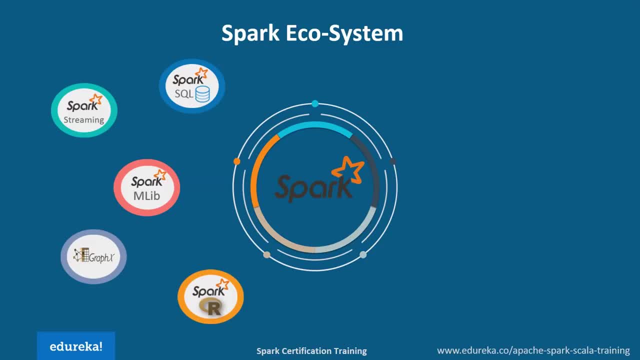 like spark SQL, spark streaming machine learning library graphics, spark are and the core API component. talking about spark SQL, It is used to leverage the power of declarative queries and optimize storage by executing SQL, like queries on spark data which is present in RDD's and other external sources. next, 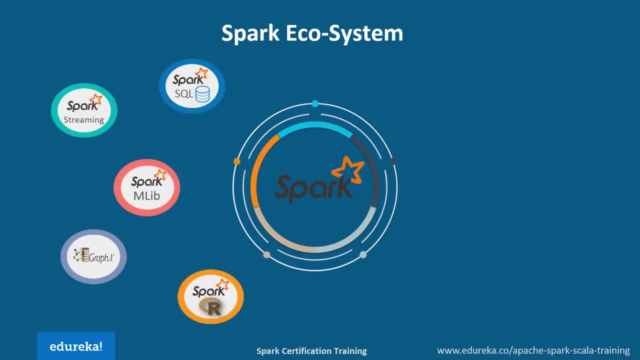 spark streaming component allows developers to perform batch processing and streaming of the data and the same application. coming to machine learning library, It eases the development and deployment of scalable machine learning pipelines, like summary statistics, cluster analysis methods, correlations, dimensionality reduction techniques, feature extractions and many more. now, graphics component lets the data scientist 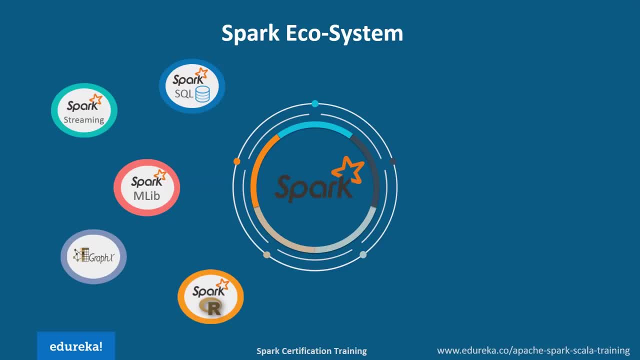 to work with graph and non graph sources to achieve flexibility and resilience in graph construction and transformation. coming to spark are. it is in our package that provides a lightweighted front end to use Apache spark. It provides a distributed data frame implementation That supports operations like selection, filtering, aggregation. 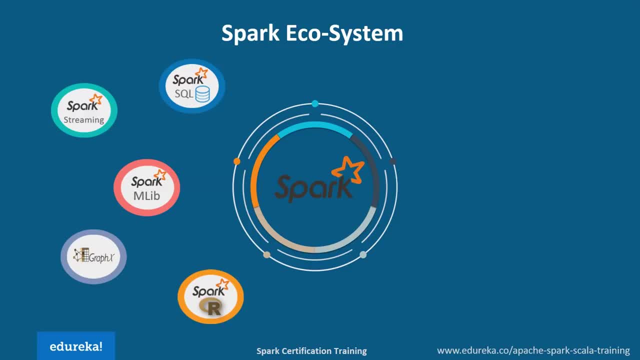 but on large data sets. It also supports distributed machine learning using machine learning library. Finally, the spark core component. It is the most vital component of spark ecosystem, which is responsible for basic IO functions, scheduling and monitoring. the entire spark ecosystem is built on the top. 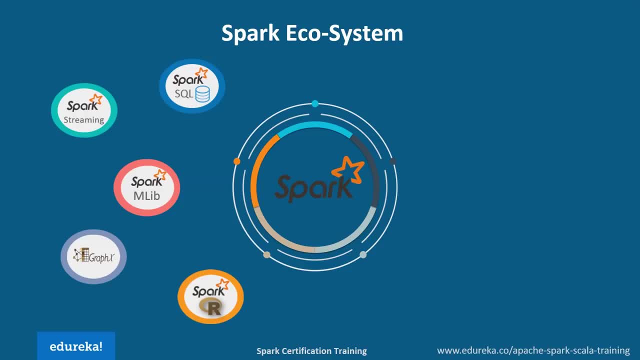 of this code execution engine, which has extensible APIs in different languages like Scala, Python are and Java. now let me tell you about the programming languages. at the first, spark support Scala- Scala as a functional programming language in which spark is written, and spark support Scala as an interface. 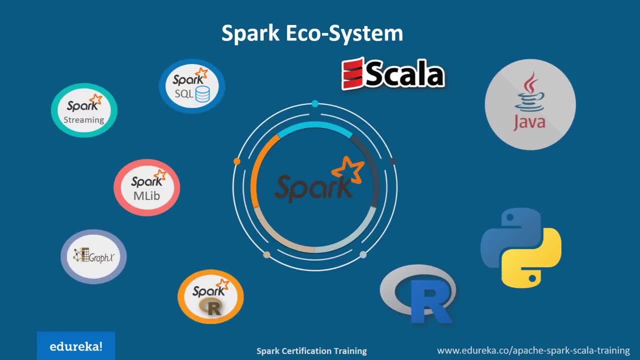 then spark also supports Python interface. You can write program in Python and execute it over the spark again, If you see the code, and Scala and Python both are very similar. then, coming to our, it is very famous for data analysis and machine learning, So spark has also added the support for our. 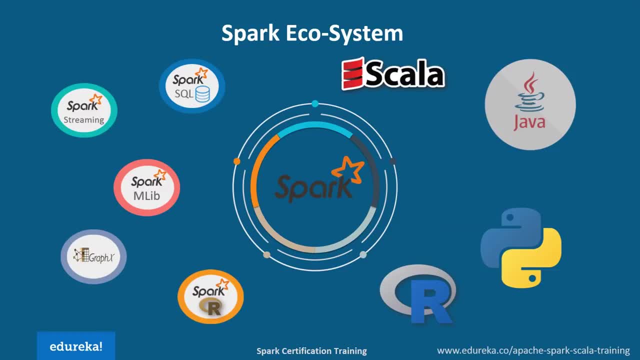 and it also supports Java, So you can go ahead and write the Java code and execute it over the spark again. Spark also provides you interactive shells for Scala Python and are very can go ahead and execute the commands one by one. So this is all about the spark ecosystem. 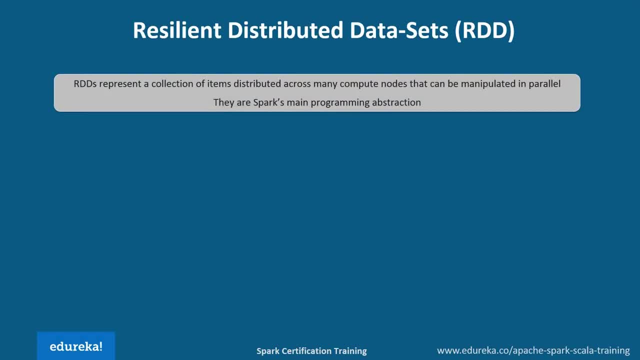 Next Let's discuss the fundamental data structure of spark. That is RDD, called as resilient distributed data sets. So in spark anything you do is around RDD. You're reading the data in spark, Then it is read into RDD again when you're transforming the data. 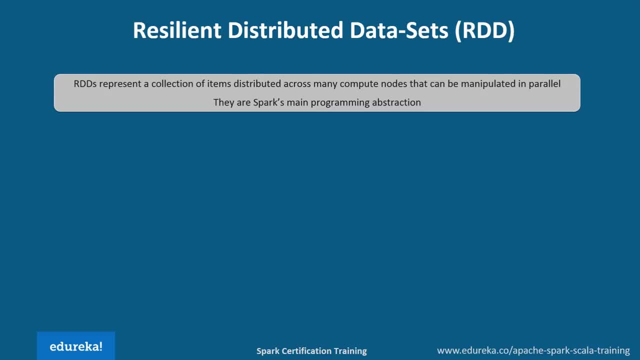 then you're performing transformations on an old RDD and creating a new one. Then at the last you will perform some actions on the data and store that data set present in an RDD to a persistent storage. resilient distributed data set is an immutable distributed collection of objects. 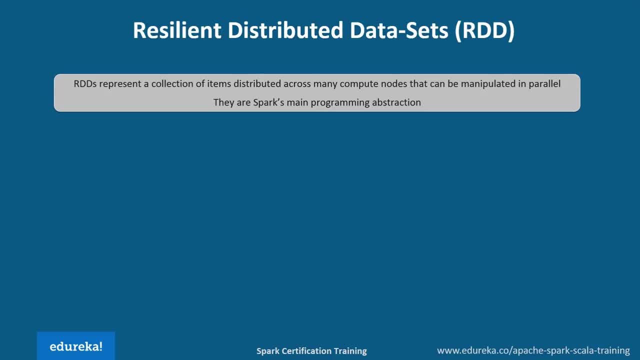 Your objects can be anything like string lines, rows, objects, collections, Etc. Now talking about the distributed environment, each data set in RDD is divided into logical partitions which may be computed on different nodes of the cluster. due to this, you can perform transformations and actions on the complete data parallelly. 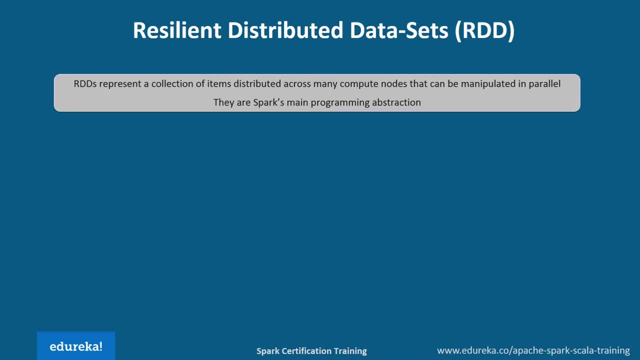 and you don't have to worry about the distribution because spark takes care of that. next, as I said, RDDs are immutable. So once you create an RDD you cannot change any content in the RDD. so you might be wondering how RDD applies those transformations. 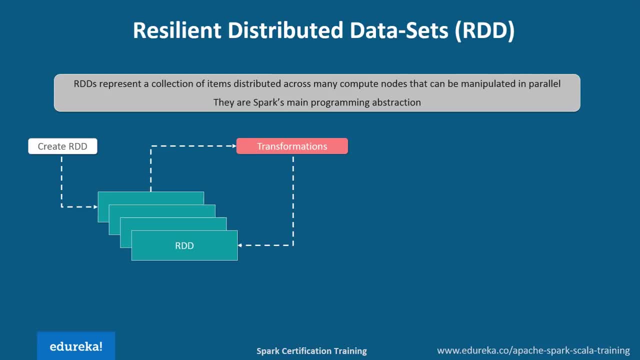 correct. when you run any transformations, a trans those transformations on old RDD and create a new RDD. This is basically done for optimization reasons. So let me tell you one thing here: RDD can be cached and persisted if you want to save an RDD for the future work. 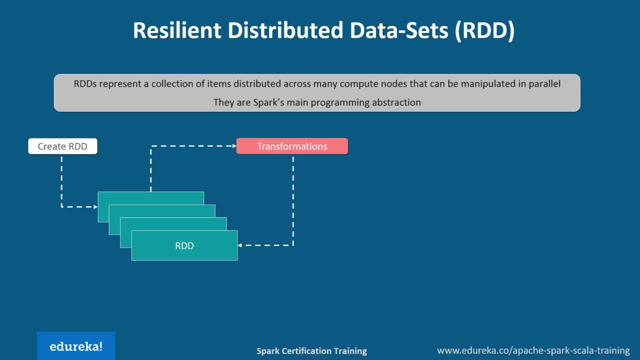 you can cash it and it will improve the spark performance. RDD is a fault-tolerant collection of elements that can be operated It on in parallel. If RDD is lost, it will automatically be recomputed by using the original transformations. This is how spark provides fault-tolerance. 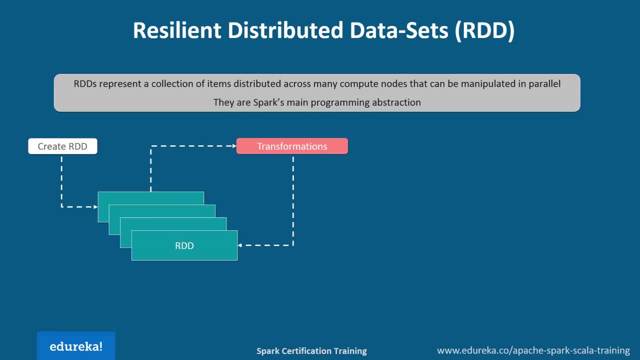 There are two ways to create RDDs: first one by parallelizing an existing collection in your driver program and the second one by referencing a data set and the external storage system, such as shared file system, HDFS, HBase, Etc. Now, transformations are the operations that you perform on RDD. 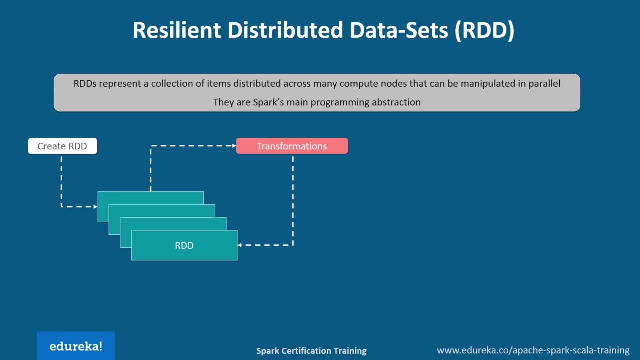 which will create a new RDD. for example, you can perform filter on an RDD and create a new RDD. Then there are actions which analyzes the RDD and produce result. simple action can be count, which will count the rows in RDD and produce a result. So I can say that transformation produce new RDD. 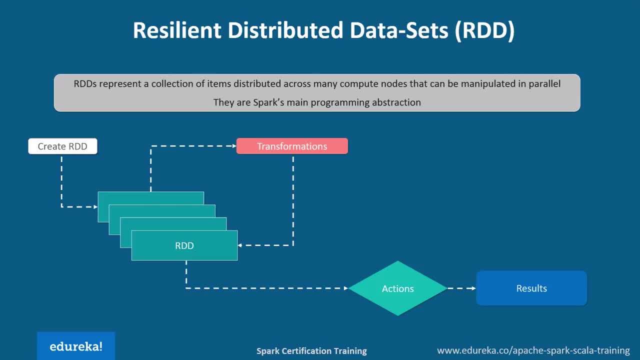 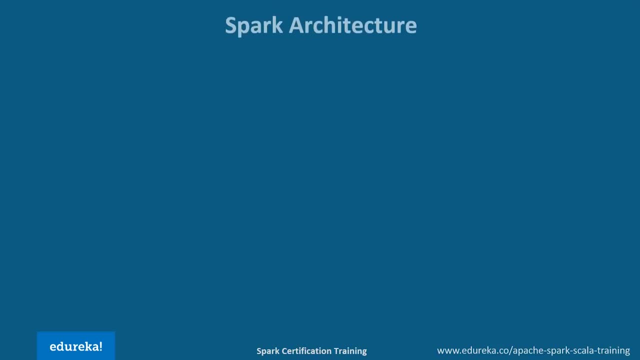 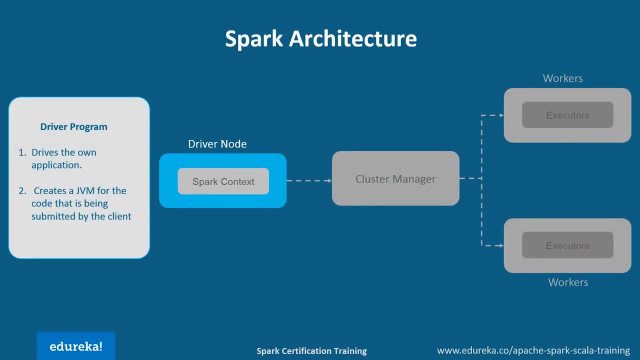 and actions produce results. So this is all about the fundamental data structure of spark, that is, RDD. Now let's dive into the core topic of today's discussion, that the spark architecture. so this is a spark architecture. in your master node, You have to drive a program which drives your application. 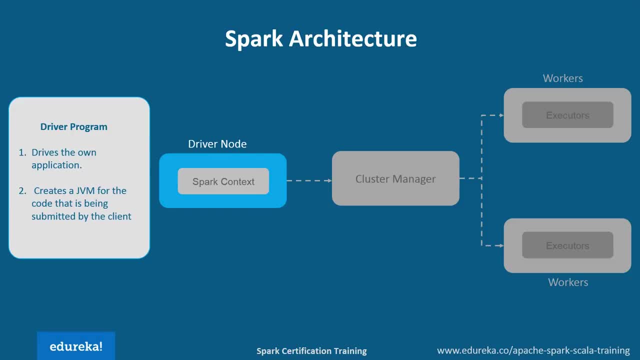 So the code that you're writing behaves as a driver program, or if you are using the interactive shell, the shell acts as a driver program inside the driver program. The first thing that you do is you create a spark context. assume that the spark context is a gateway. 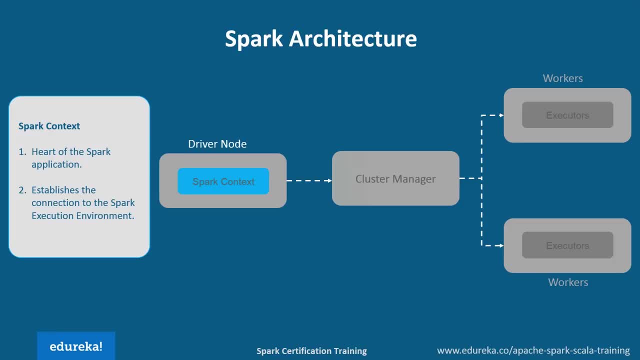 to all spark functionality at the similar to your database connection. So any command you execute in your database goes through the database connection. Similarly, anything you do on spark goes through the spark context. Now this spark context works with the cluster manager to manage various jobs: the driver program. 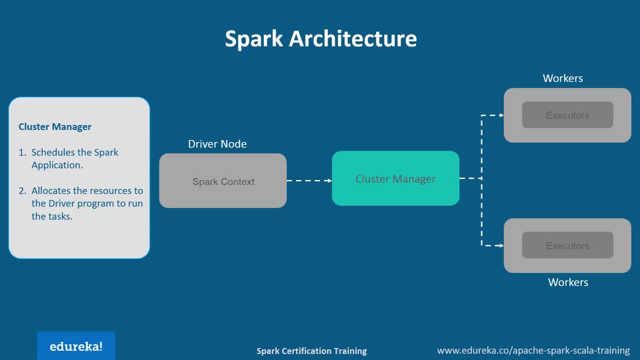 and the spark context takes care of executing the job across the cluster. a job is split into the tasks and then these tasks are distributed over the worker node. So anytime you create a RDD in the spark context, that RDD can be distributed across various nodes and can be cached there. 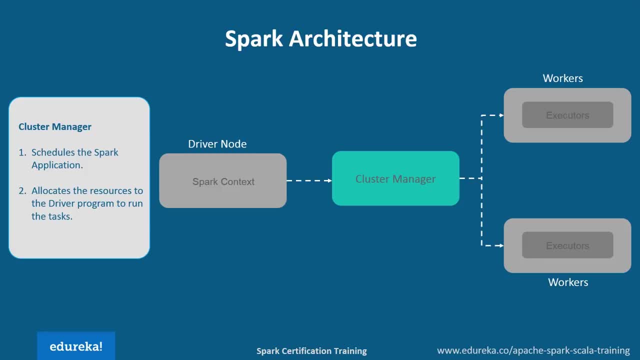 So RDD is set to be taken, partitioned and distributed across various nodes. Now worker nodes are the slave nodes whose job is to basically execute the tasks. the task is then executed on the partition RDDs in the worker nodes and then returns the result back to the spark context. 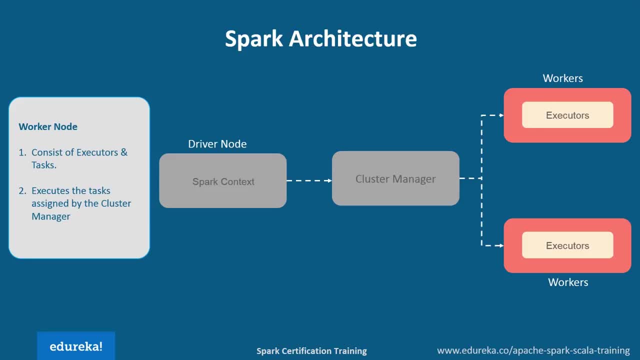 spark context takes the job, breaks the job into the task and distribute them on the worker nodes, and these tasks works on partition RDDs, perform whatever operations you wanted to perform and then collect the result and give it back to the main spark context. If you increase the number of workers, 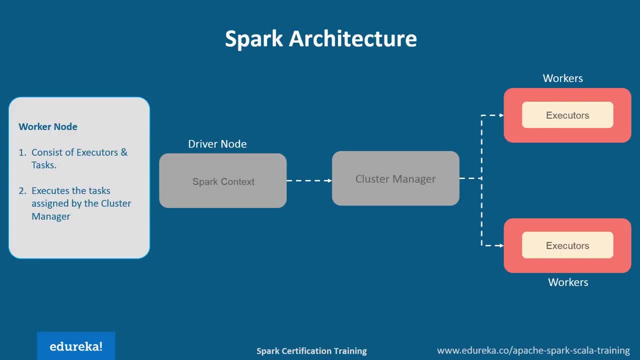 then you can divide jobs and more partitions and execute them badly over multiple systems. This will be actually a lot more faster. Also, if you increase the number of workers, it will also increase your memory and you can cache the jobs so that it can be executed much more faster. 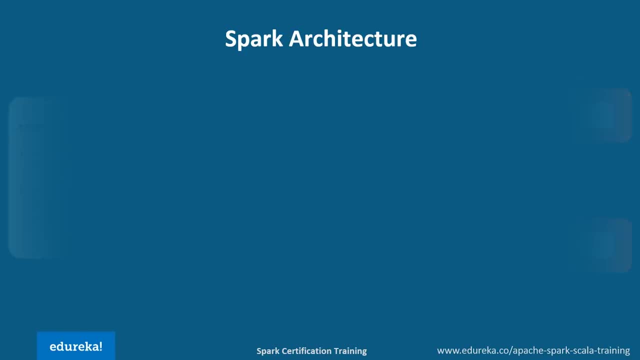 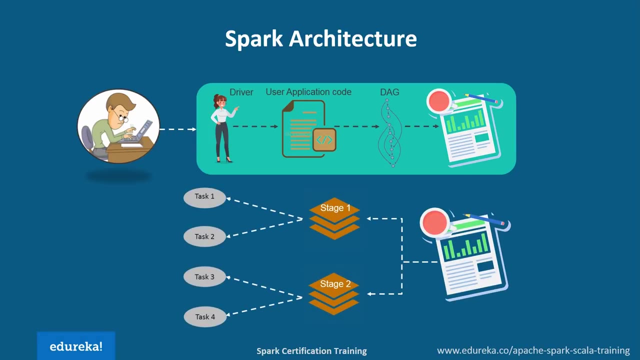 So this is all about spark architecture. Now let me give you an infographic idea about the spark architecture. It follows master slave architecture. here The client submits spark user application code. when an application code is submitted, driver implicitly converts a user code that contains transformations and actions. 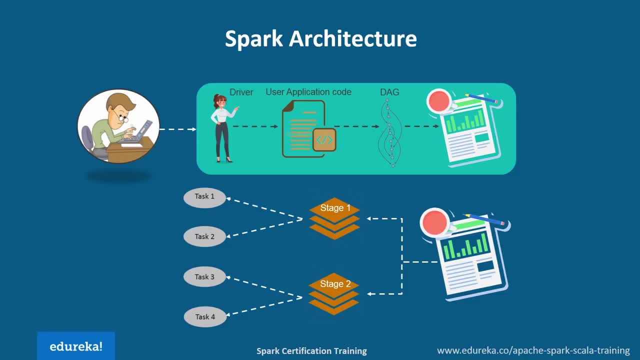 into a logically directed graph called DHE. at this stage It also performs optimizations such as pipe planning transformations. Then it converts a logical graph called DHE into physical execution plan with many stages. after converting into physical execution plan, It creates a physical execution units called tasks. 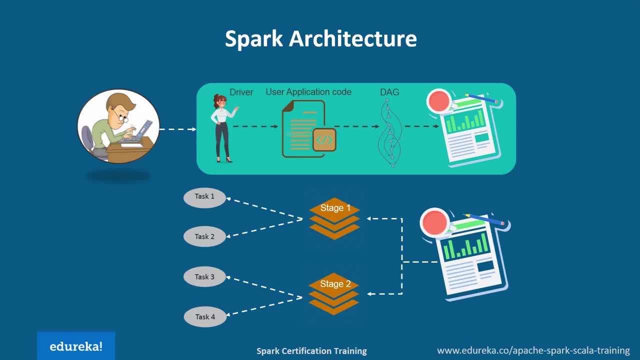 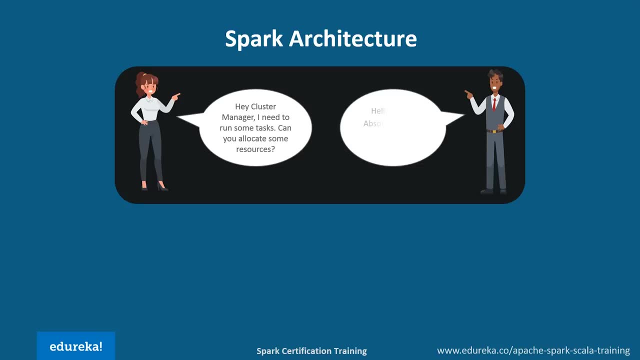 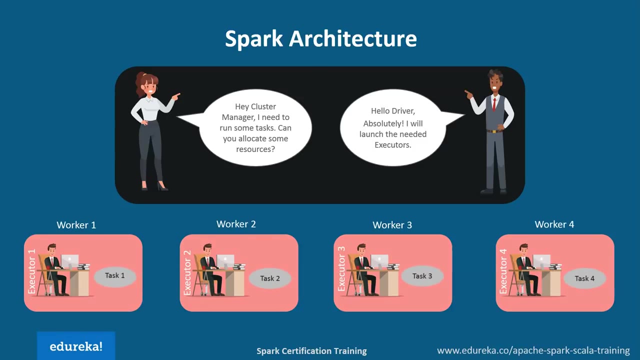 under each stage. Then these tasks are bundled and sent to the cluster. Now driver talks to the cluster manager and negotiates the resources, and cluster manager launches the needed executors. at this point, driver will also send the task to the executors based on the placement. 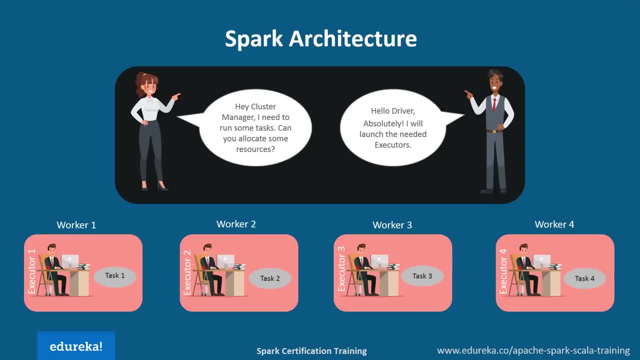 when executors start to register themselves with the drivers so that driver will have a complete view of the executors and executors now start executing the tasks that are assigned by the driver program. at any point of time when the application is running, driver program will monitor. 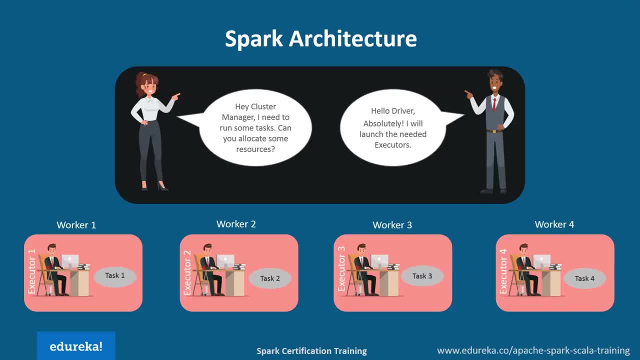 the set of executors that runs and the driver node also schedules a future task based on data placement. So this is how the internal working takes place. in spark architecture There are three different types of workloads that spark and cater first, batch mode. in case of batch mode, 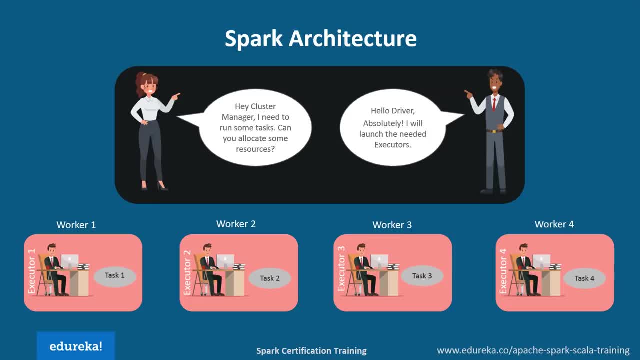 We run a bad job here. You write a job and then schedule it. it works through a queue or batch of separate jobs through manual intervention. next, interactive mode. This is an interactive shell where you go and execute the commands one by one. So you will execute one command, check the result. 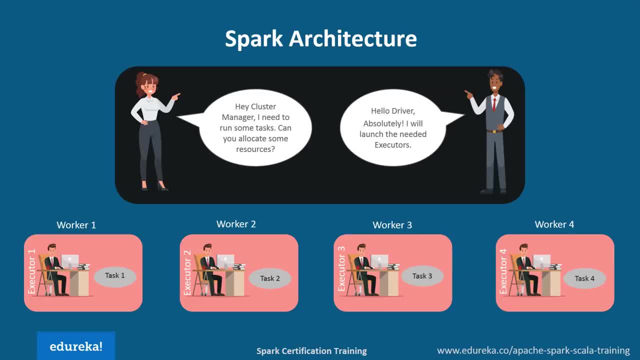 and then execute the other command based on the output result, and so on. it works similar to the SQL shell, So shell is the one which executes a driver program, So it is generally used for development work, or it is also used for ad hoc queries. then comes the streaming mode. 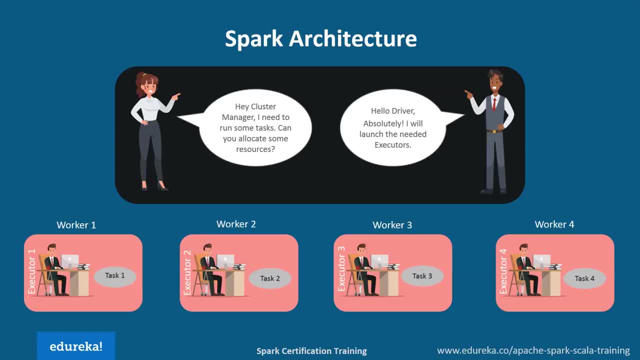 where the program is continuously running, as in when the data comes. it takes the data and do some transformations and actions on the data and then produce output results. So these are the three different types of workloads that spark actually caters. now let's move ahead and see a simple demo here. 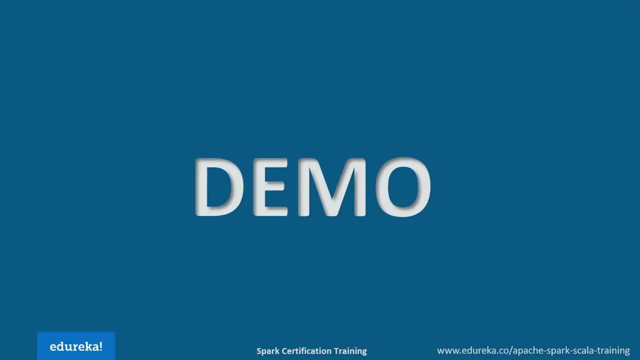 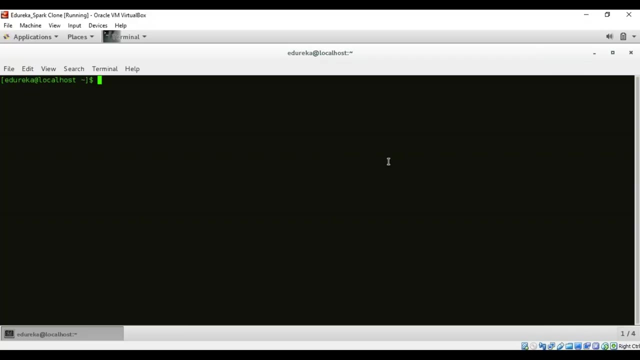 Let's understand how to create a spark application and spark shell using Scala. So let's understand how to create a spark application in spark shell using Scala. assume that we have a text file in the HDFS directory and we are counting the number of words in that text file. 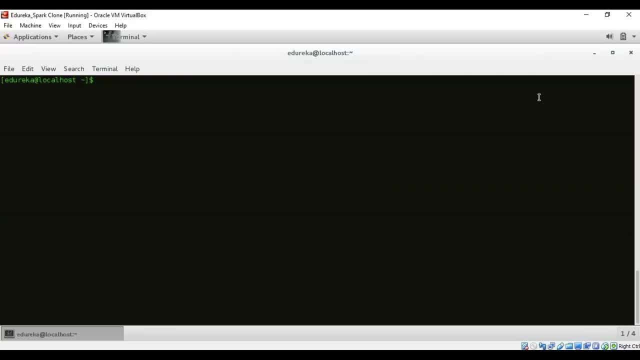 So let's see how to do it. So before I start running, let me first check whether all my demons are running or not. So I'll type pseudo GPS: So all my spark demons and Hadoop demons are running, that I have, master worker, a spark demons. 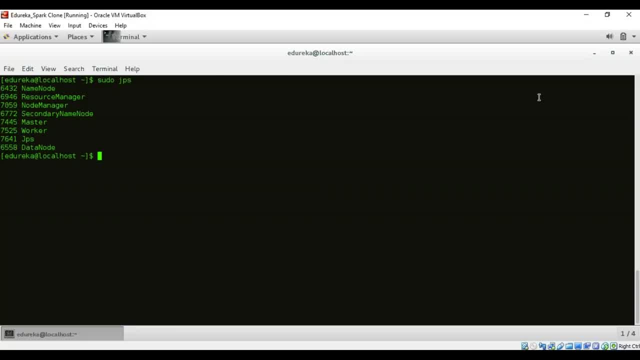 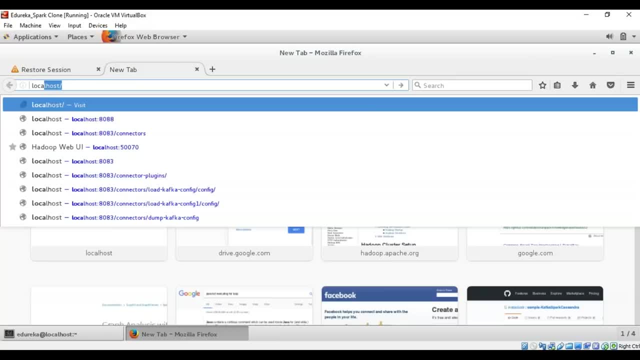 and name no resource manager, node manager, everything as Hadoop demons. So the first thing that I do here is I run the spark shell. So it takes bit time to start and the main while let me tell you, the web UI port for spark shell is localhost 4040.. 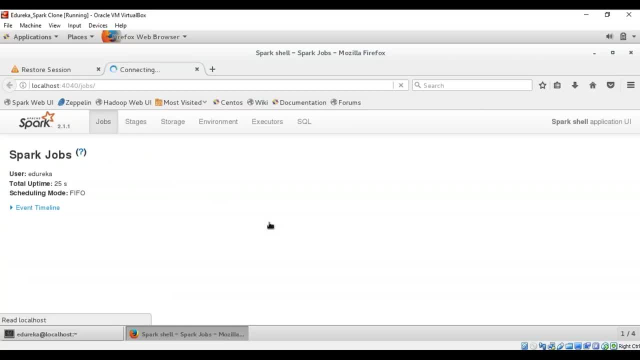 So this is a web UI for spark, like if you click on jobs right now we have not executed anything, So there is no details over here. So they have job stages. So once you execute the jobs, if you'll be having the records of the task. 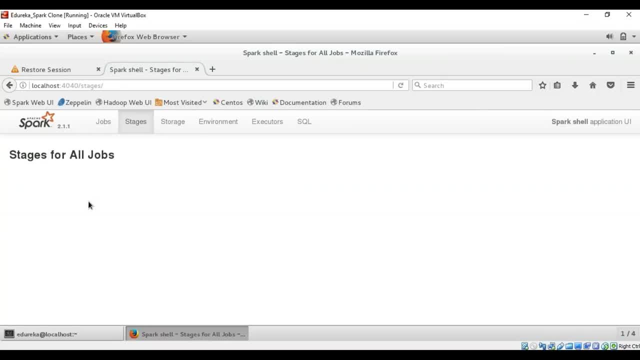 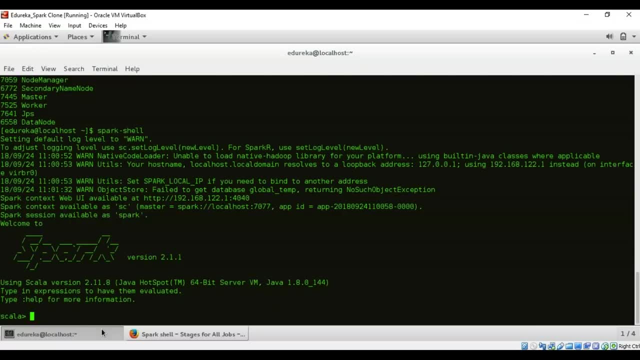 that you have executed here. So here you can see the stages of various jobs and tasks executed. So now let's check whether our spark shell has started or not. Yes, So you have your spark version as 2.1.1 and you have a scholar shell over here. 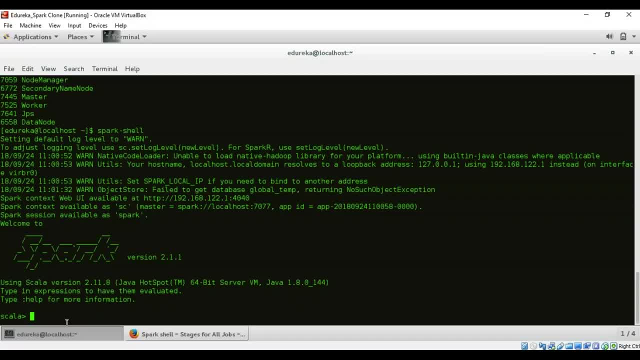 So before I start the code, let's check the content that is present in the input text file by running this command. So I'll write where test is equal to SC dot text file, because I have saved a text file over there and I'll give the HDFS path location. 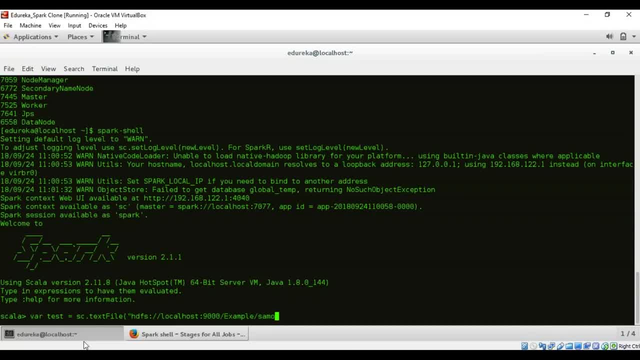 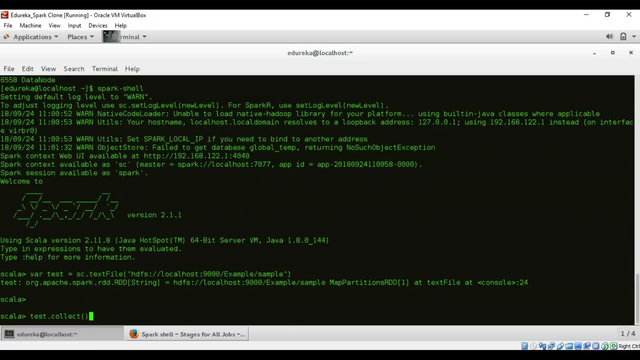 I've stored my text file in this location And sample is the name of the text file. So now let me give test dot collect so that it collects the data and displays the data that is present in the text file. So in my text file, 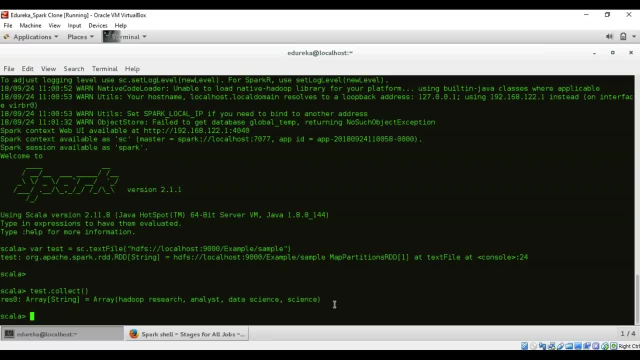 I have Hadoop research analyst data, signs and signs, So this is my input data. So now let me map the functions and apply the transformations and actions. So I'll give var map is equal to SC dot text file And I will specify my input path location. 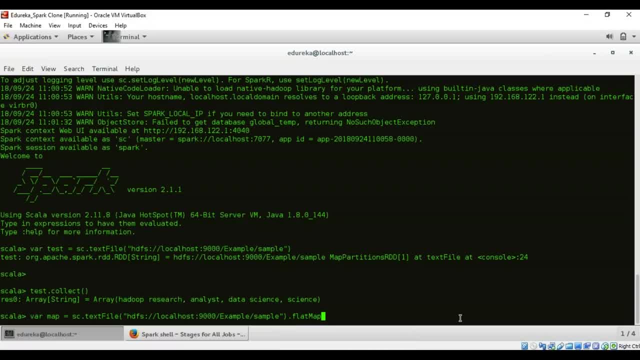 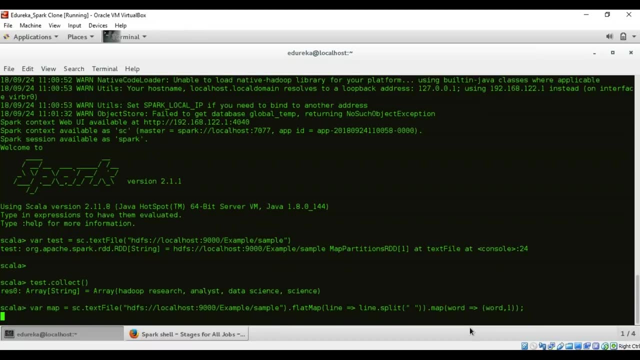 So this is my input path location and I'll apply the flat map transformation to split the data That is separated by space and then map the word count to be given as word comma one. Now this will be executed. Yes, Now let me apply the action for this to start. 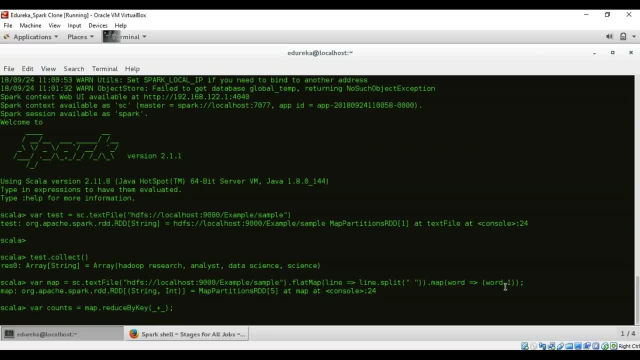 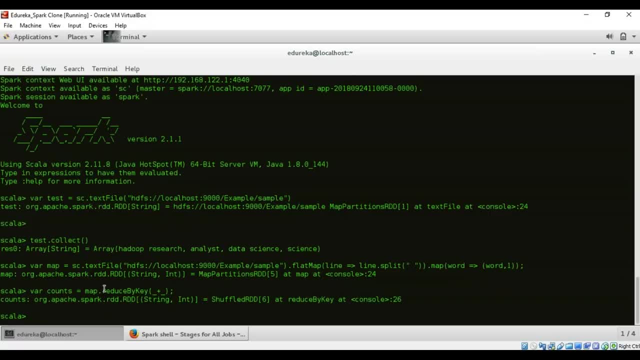 The execution of the task. So let me tell you one thing here before applying an action: The spark will not start the execution process. So here I have applied reduced by key as the action to start counting the number of words in the text file. 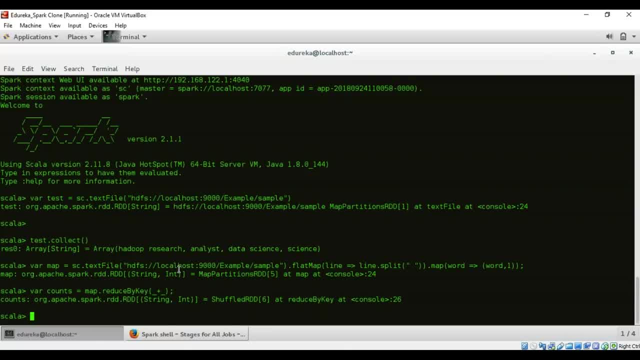 So now we are done with applying transformations and actions as well. So now the next step is to specify the output location, to store the output file. So I'll give us counts dot, save as text file and then specify the location for my output file. 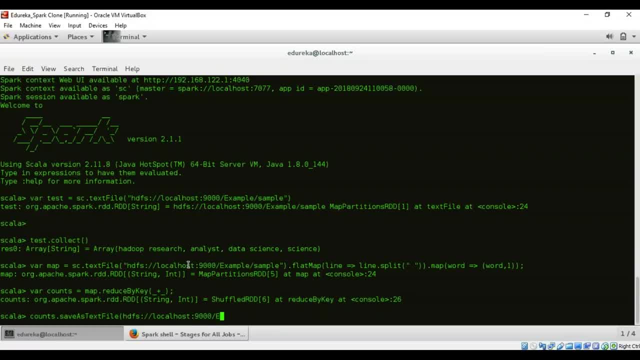 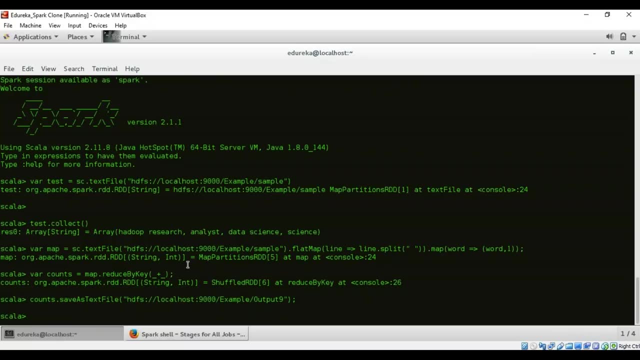 I'll store it in the same location where I have my input file, and I will specify my output file name as output 9- cool. I forgot to give a double quotes And I will run this, So it's completed now. So now let's see the output. 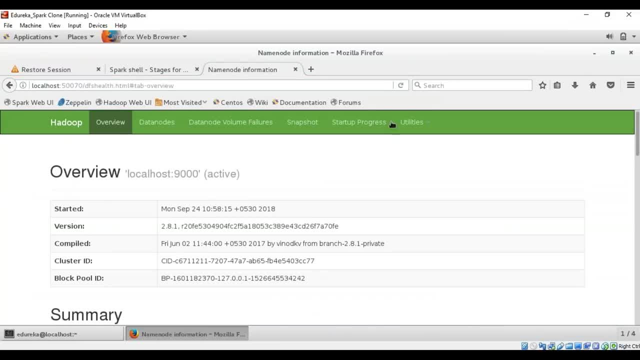 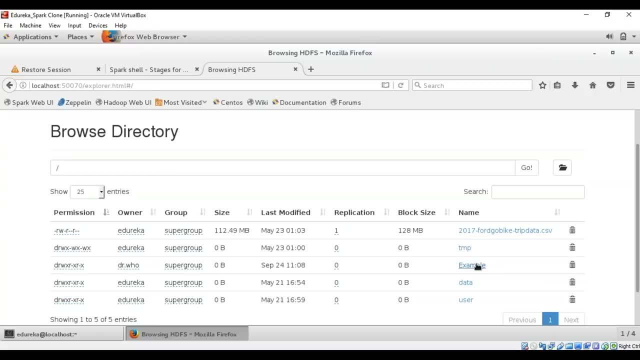 I will open my Hadoop web UI by giving localhost 50070 and browser file system to check the output. So, as I have said, I have example as my directory that I have created and in that I have specified output 9 as my output. 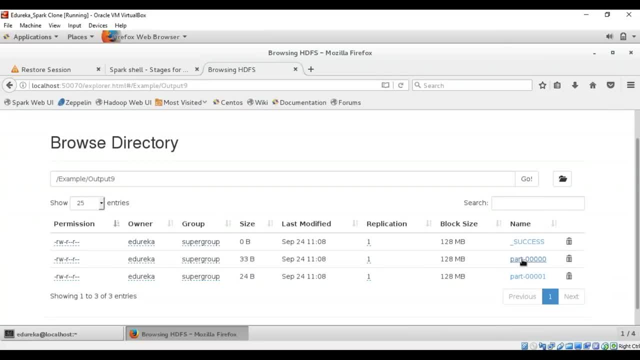 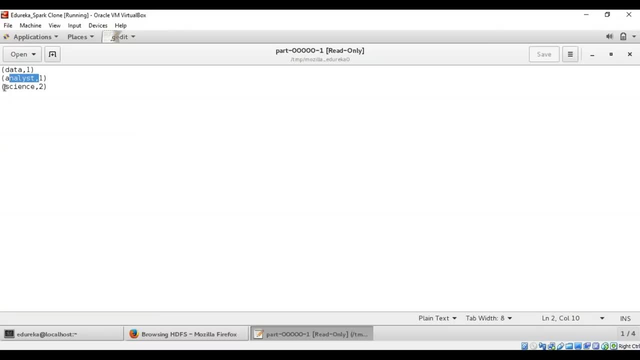 So I have the two part files being created. Let's check each of them one by one. So we have: the data count as one, analyst count as one and science count as two. So this is a first part file. Now let me open the second part file for you. 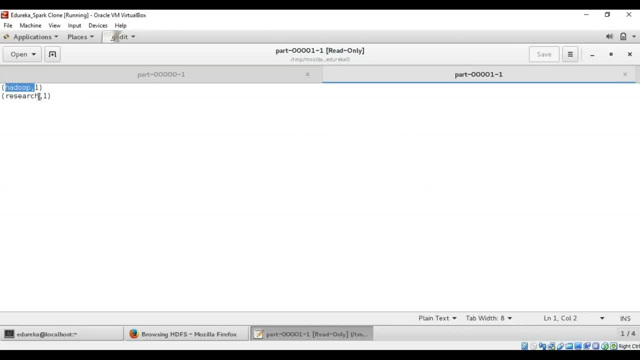 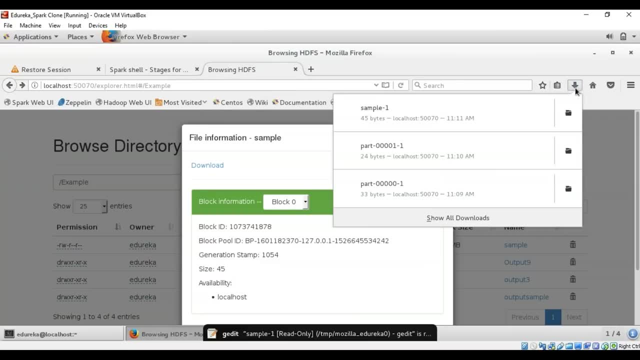 So this is the second part file, where you have Hadoop count as well and the research count as one. So now let me show you the text file that we have specified as the input. So, as I have told you, Hadoop count is one research count. 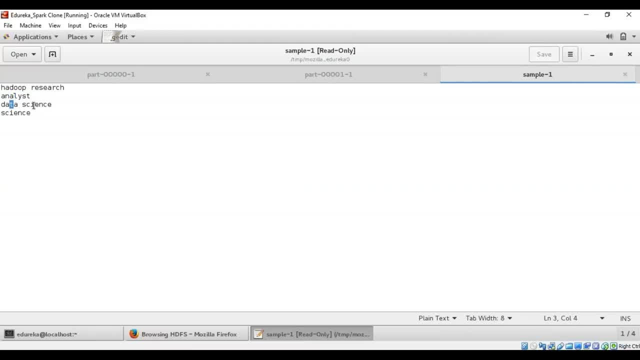 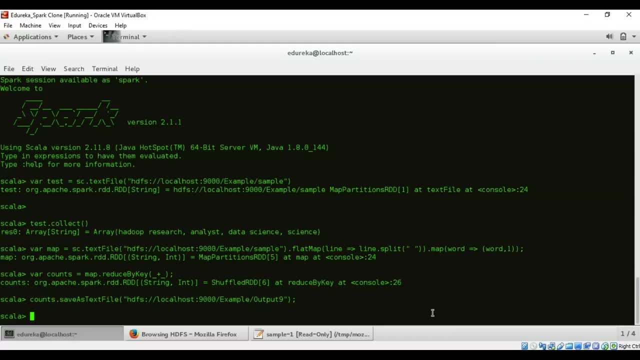 is one analyst, one data one, science and science as one one. So you might be thinking data science is a one word. No, in the program code We have asked to count the word that is separated by a space, So that is why we have science count as two. 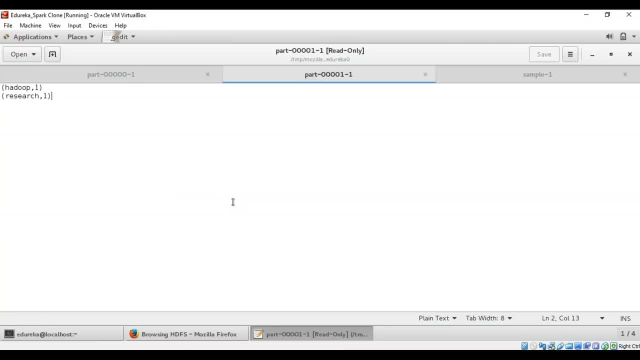 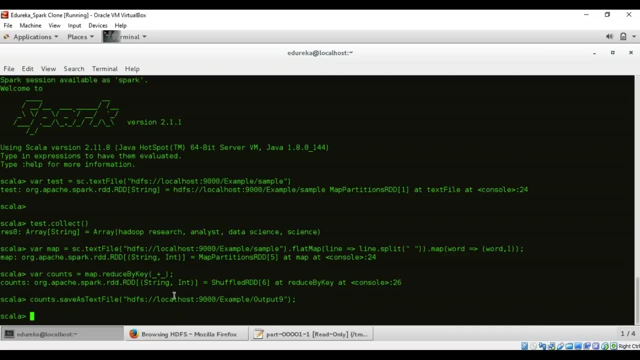 I hope you got an idea about how word count works. Similarly, I will now parallelize 1 to 100 numbers and divide the task into five partitions to show you what is partitions of task. So I will write: SC dot. parallelize 1 to 100 numbers. 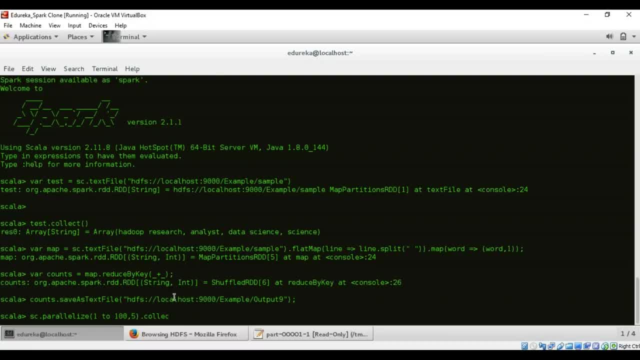 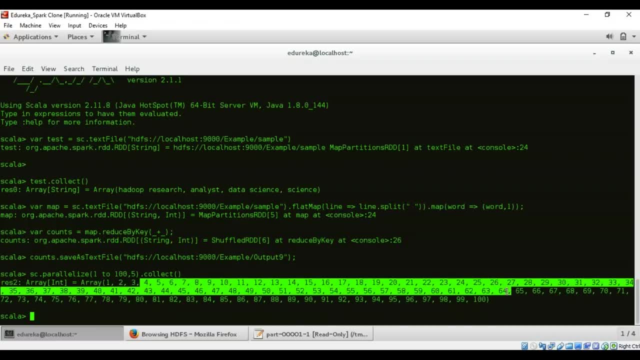 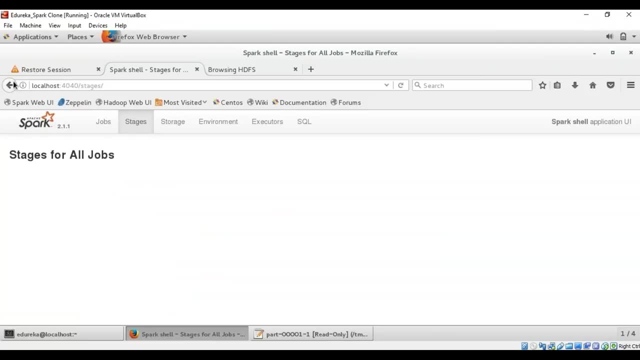 and divide them into five partitions and apply collect action to collect the numbers and start the execution. So it displays you an array of 1 to 100 numbers. Now let me explain You the job, stages, partitions, even timeline, dag, representation and everything. 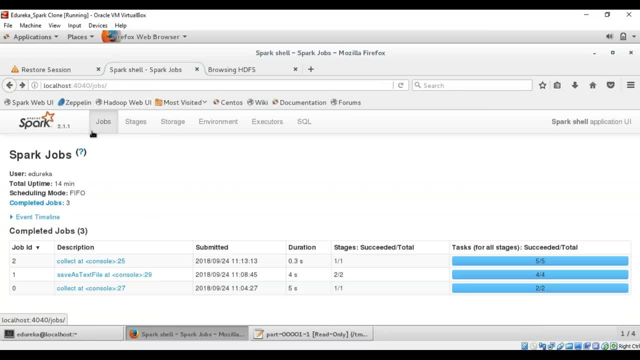 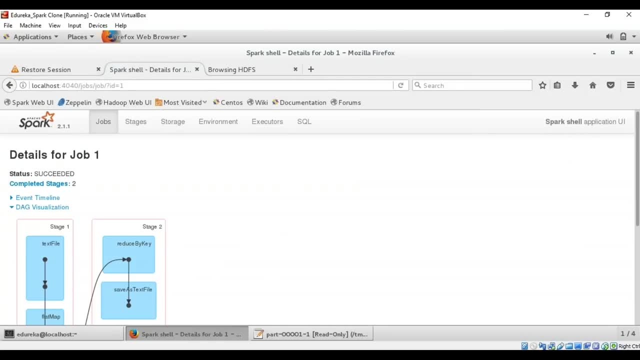 So now let me go to the web UI of spark and click on jobs. So these are the tasks that have submitted. So coming to word count example. So this is the DAG visualization. I hope you can see it clearly. first You collected the text file, then you applied flat map transformation. 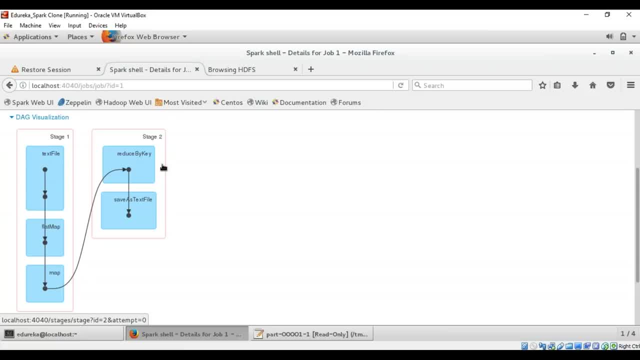 and mapped it to count the number of words and then applied, reduce by key action And then save the output file as save as text file. So this is the entire tag visualization of the number of steps that we have covered in a program. So here it shows the completed stages. that is, two stages. 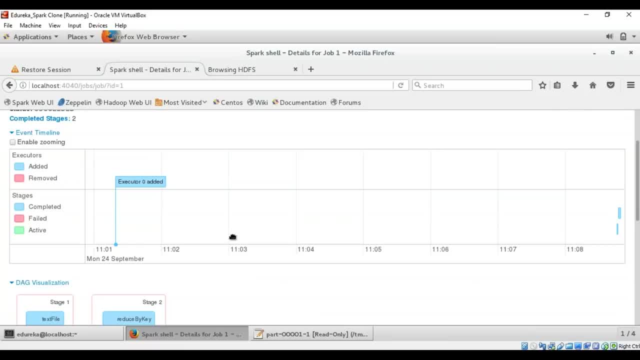 and it also shows the duration. that is two seconds, And if you click on the event timeline, it just shows the executor that is added, and in this case you cannot see any partitions because you have not split the jobs into various partitions. So this is how you can see. 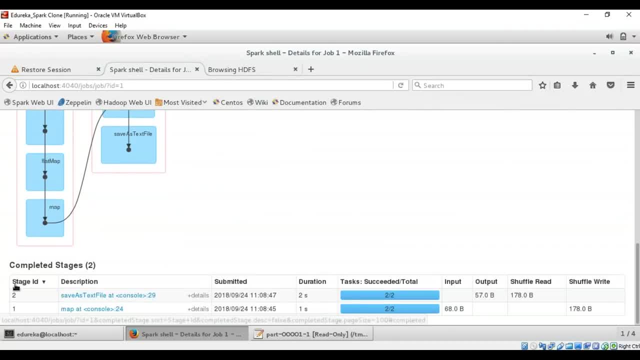 The event timeline and the DAG visualization. here You can also see the stage ID descriptions when you have submitted that. I have just submitted it now and in this it also shows the duration that it took to execute the task and the output bytes that it took. the shuffle read shuffle. 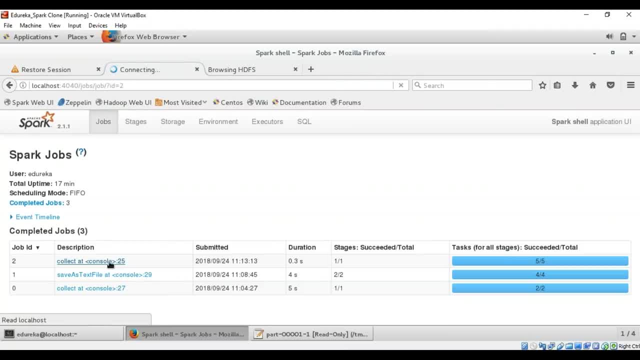 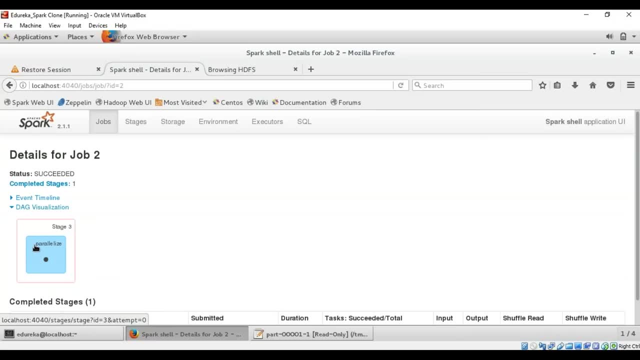 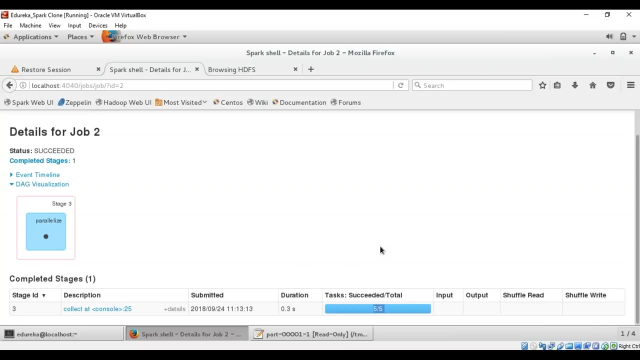 right and many more. now to show you the partitions: see, in this you just applied SC dot parallelize right. So it is just showing one stage where you have applied the parallelize transformation. Here it shows the succeeded task as five by five, that is, you have divided the task into five stages. 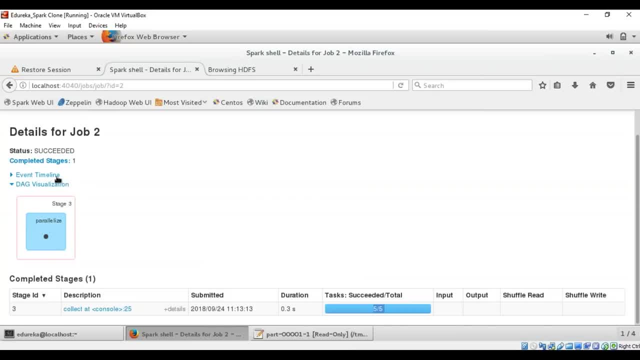 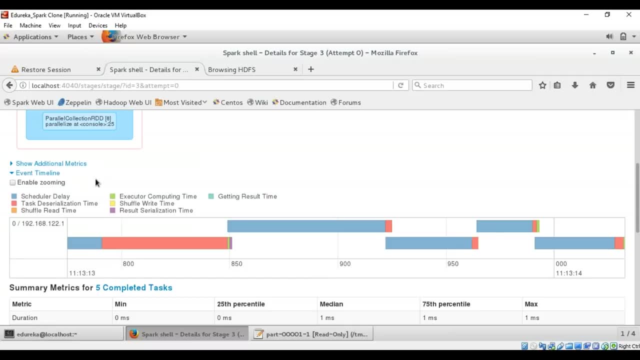 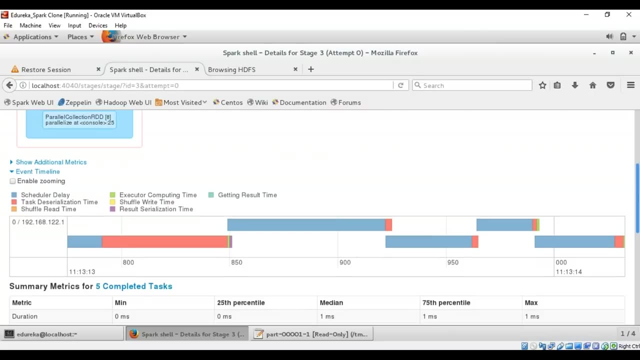 and all the five stages has been executed successfully. Now here you can see the partitions of the five different stages that is executed in parallel. So depending on the colors it shows the scheduler, delay, the shuffle rate, time, executor, computing time, results realization time and getting result time and many more. so you can see. 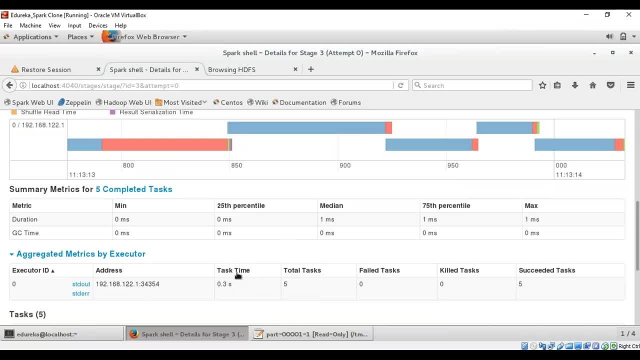 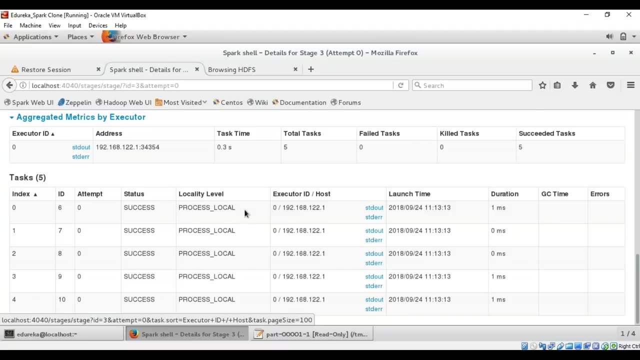 the duration that it took to execute the five tasks in paddle at the same time as maximum one milliseconds. So in memory, spark has much faster computation and you can see the IDs of all the five different tasks. All our success. you can see the locality level. you can see. 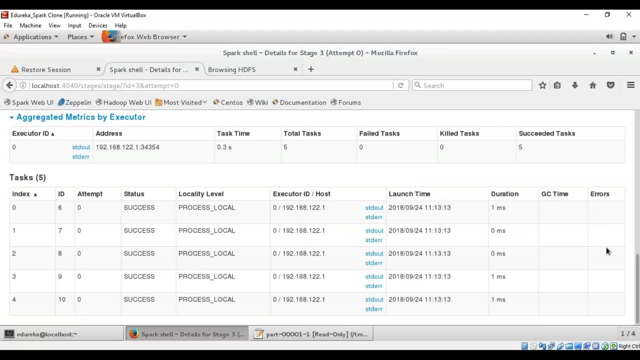 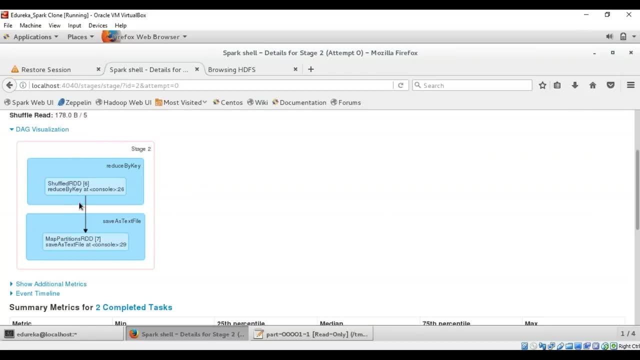 the executor and the host, IP ID, the launch time, the duration- it take everything. so you can also see that we have created RDD and parallelized it. similarly here also for word count example, You can see the RDD that has been created and also the actions that you have applied. 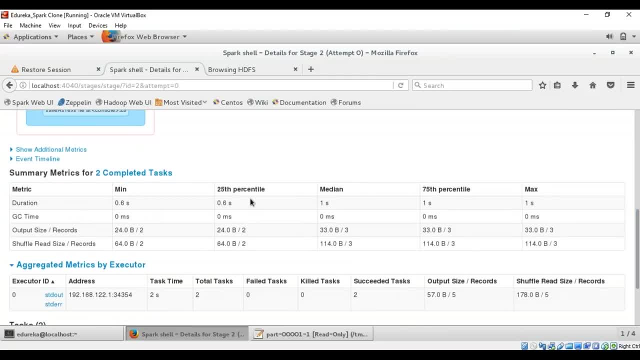 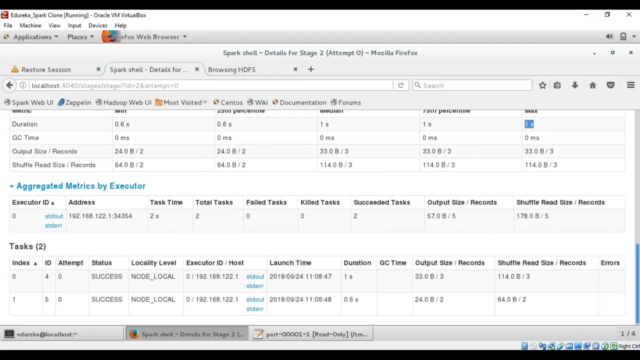 to execute the task and you can see the duration that it took. even here Also, it's just one millisecond that it took to execute the entire word count example and you can see the ID is locality level executor ID. So in this case, 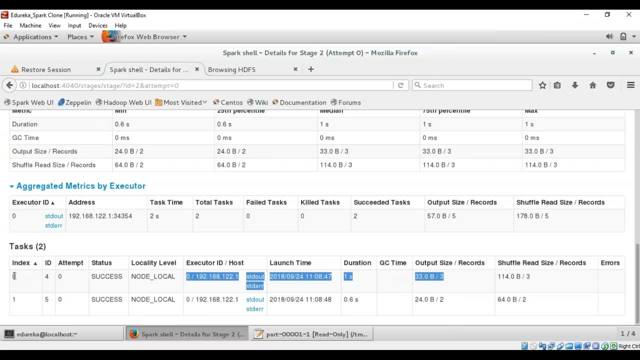 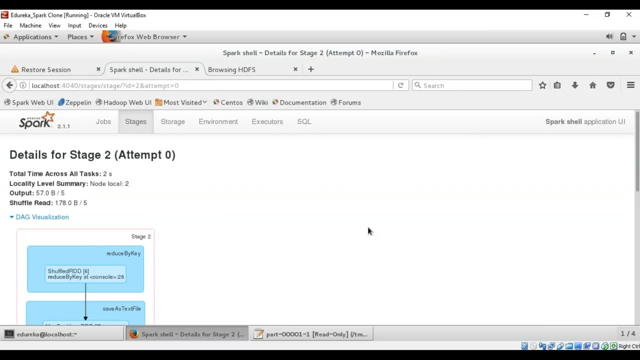 we have just executed the task in two stages, So it is just showing the two stages. So this is all about how web UI looks and what are the features and information that you can see, And the web UI of spark after executing the program and the scholar shell. 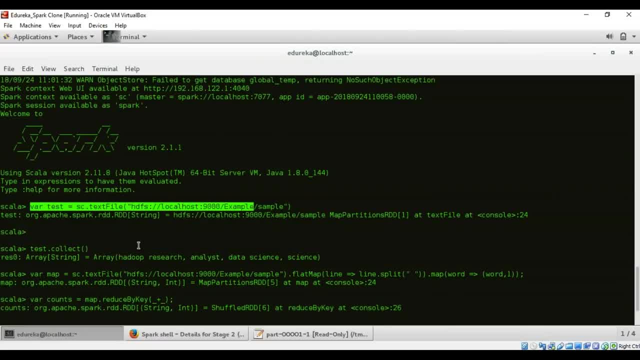 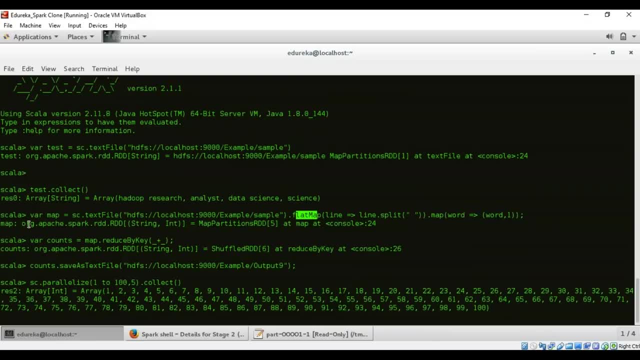 So in this program you can see that first we gave the path to the input location and check the data that is presented in the input file, and then we applied flat map transformations and created RDD and then applied action to start the execution of the task and save the output file in this location. 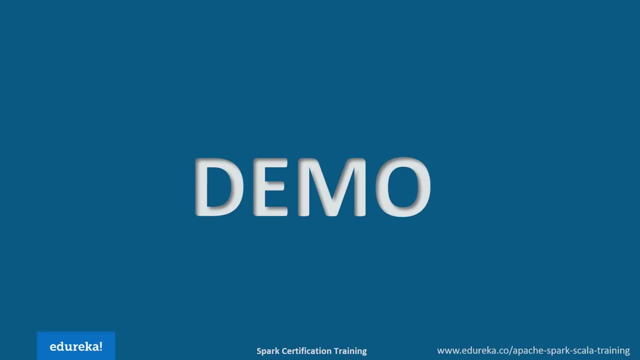 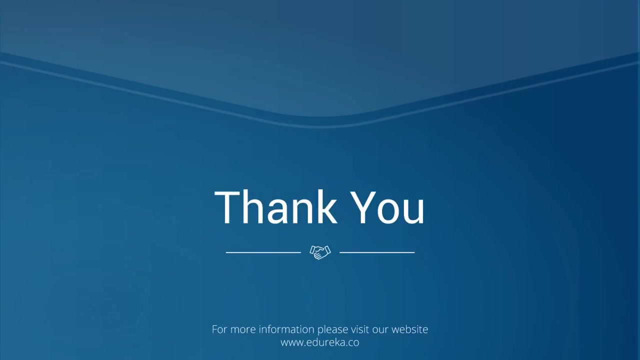 So I hope you got a clear idea of how to execute a word count example and check for the various features and spark web UI like partitions that visualizations and everything. I hope you found the session interesting. That's all for the session. Thank you and have a nice day. 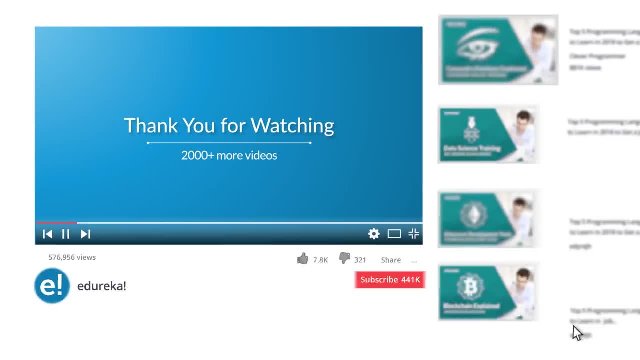 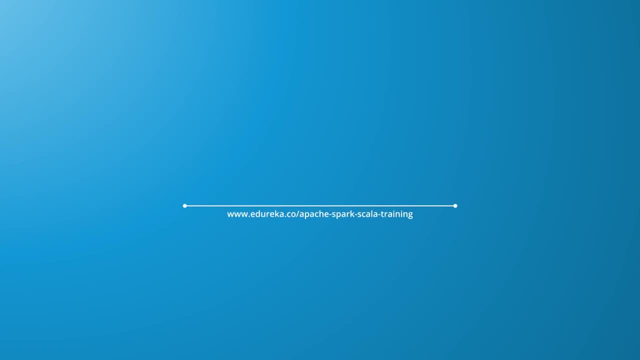 I hope you have enjoyed listening to this video. Please be kind enough to like it and you can comment any of your doubts and queries and we will reply them at the earliest. Do look out for more videos in our playlist and subscribe to Edureka channel to learn more. Happy learning, Thank you.